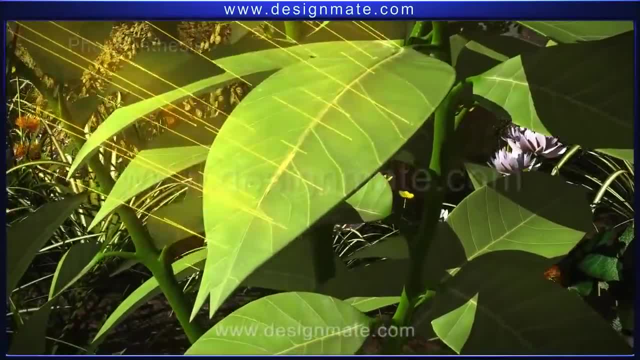 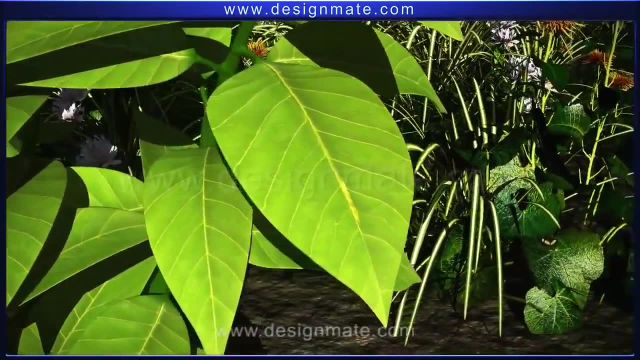 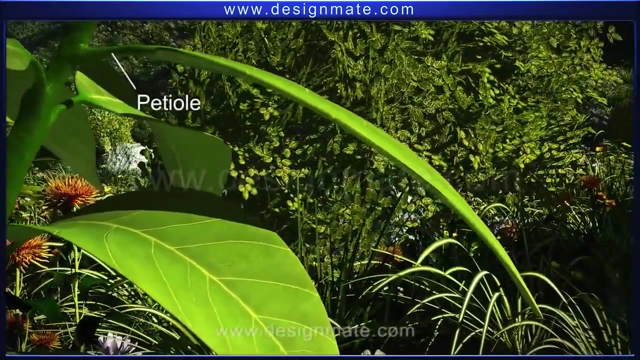 A look at nature is an absolute treat to our senses. A leaf is a very important part of the plant. Photosynthesis, the ultimate provider of food and oxygen, occurs in the leaf. A leaf consists of a flat, thin lamina which is joined to the stem by a petiole. 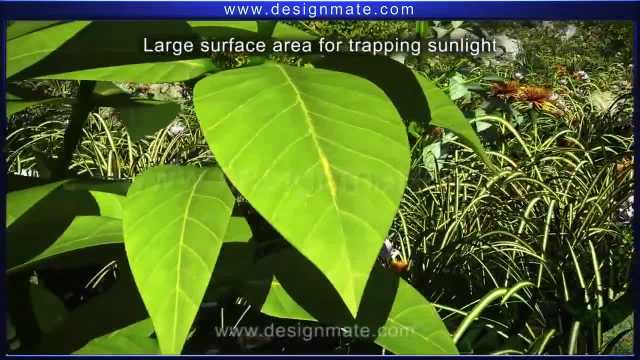 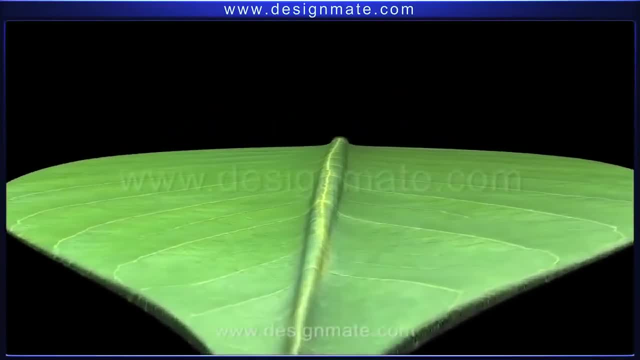 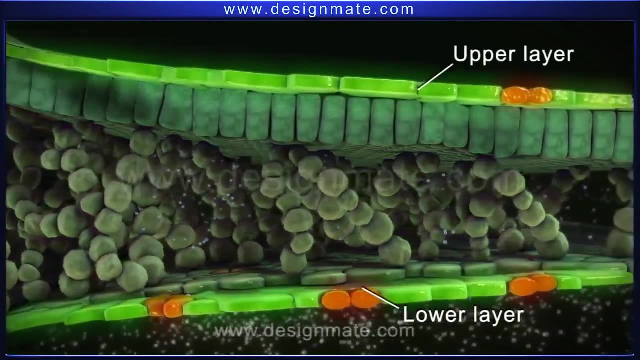 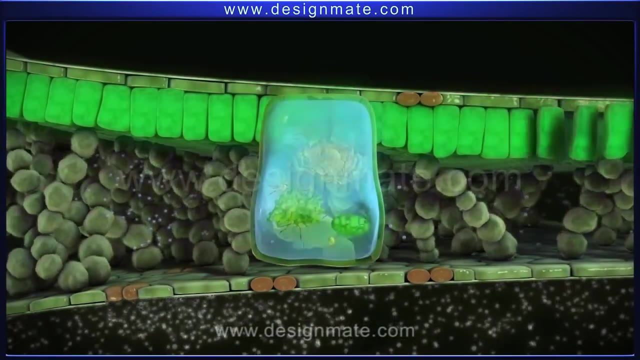 The flattened lamina provides large surface area for trapping sunlight. A cross-section of the leaf shows the upper and lower layers of cells, which are flat and irregular. Below the upper layer is the layer of tightly packed cells. These cells have specialized organelles called chloroplasts. 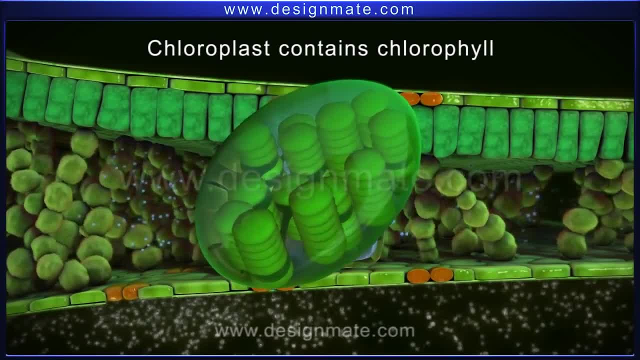 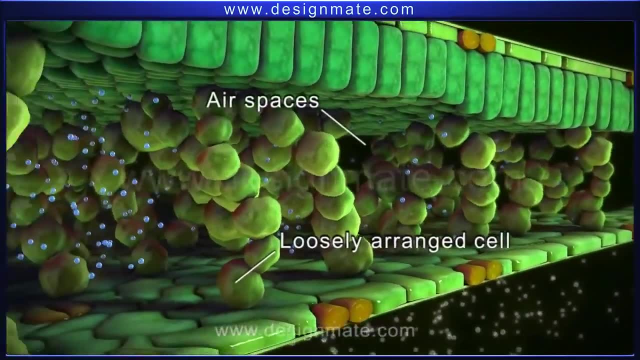 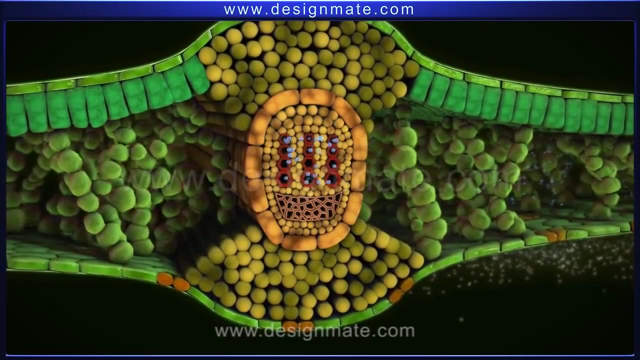 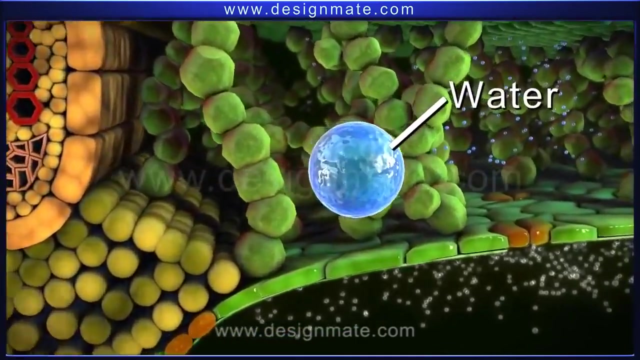 Chloroplasts contain the pigment chlorophyll, which gives the green color to the leaf. The next layer has loosely arranged cells with large air spaces. The section also shows tubes specific for transporting the absorbed water into the leaves. The lower layer has many pores, called stomata. 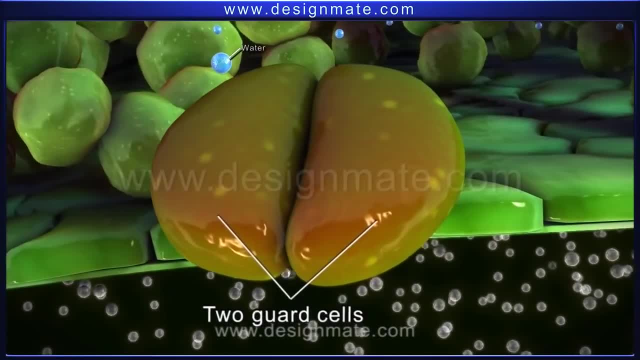 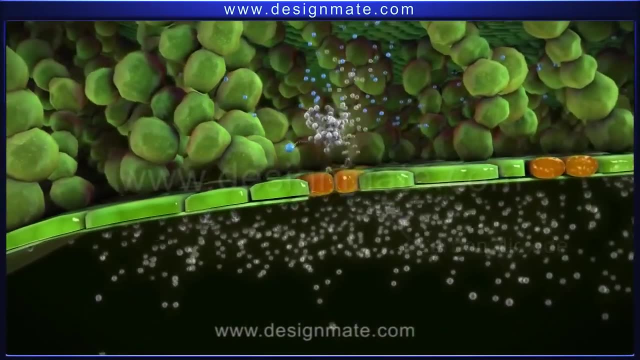 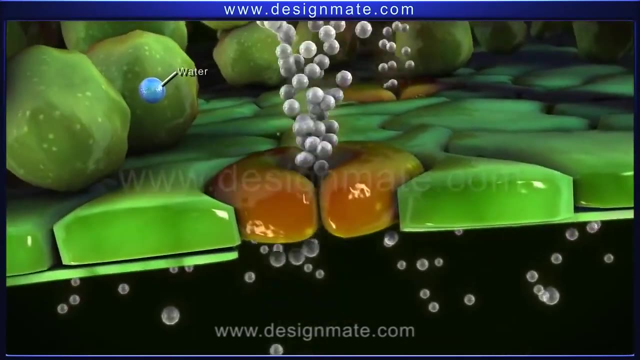 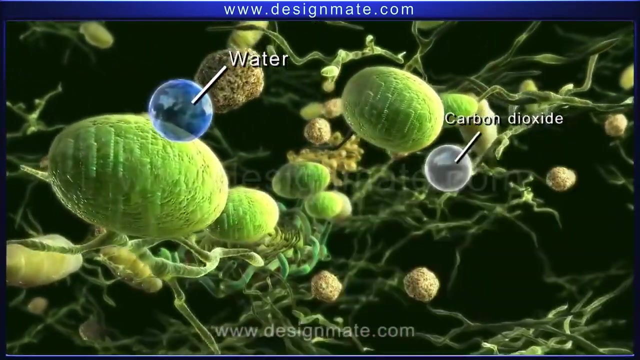 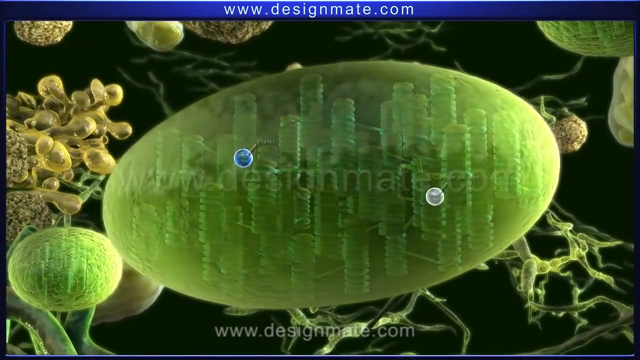 Each stoma is surrounded by two guard cells which regulate opening and closing of the stomata. A leaf absorbs carbon dioxide from the environment through these stomata which, after passing through air spaces, enter into the chlorophyll-containing cells. Both water and carbon dioxide molecules are finally absorbed by the chloroplast. 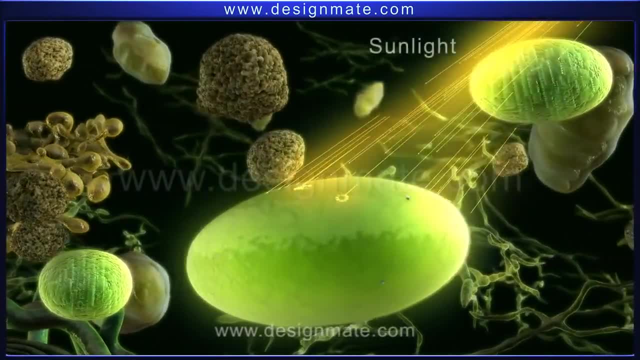 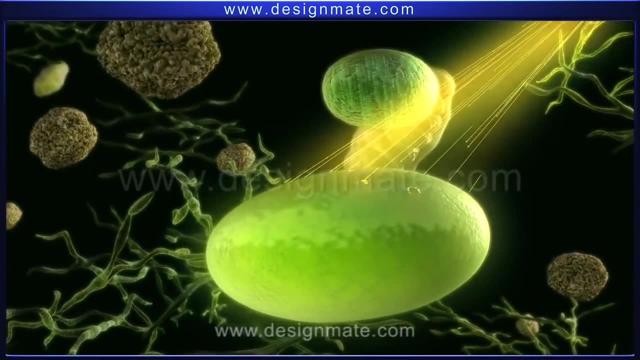 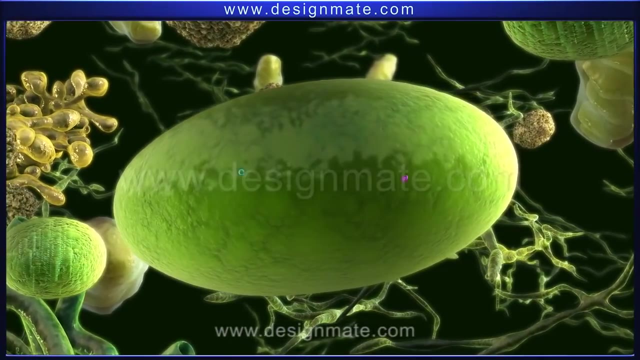 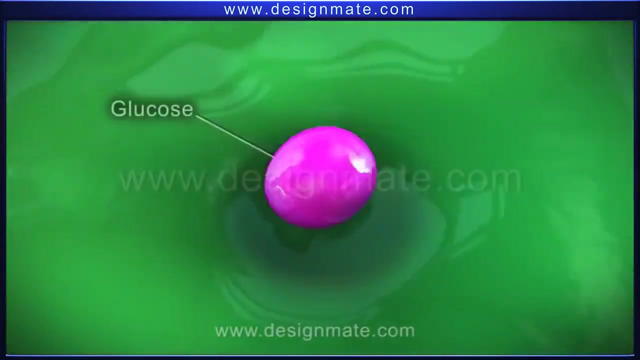 These chlorophyll cells are components of the leaf's tissue. Chloroplasts also have the capacity for trapping energy from sunlight, and this energy is used to synthesize glucose and oxygen from carbon dioxide in water. These oxygen and glucose molecules diffuse out of the chloroplast. 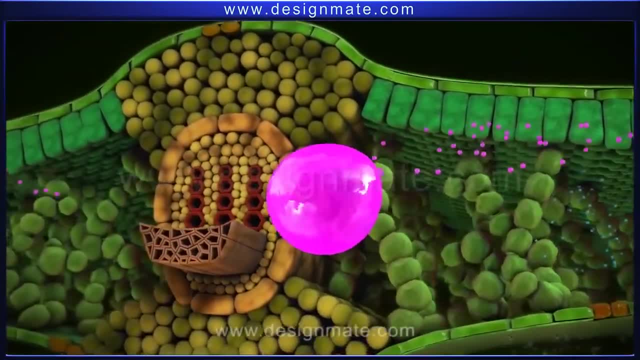 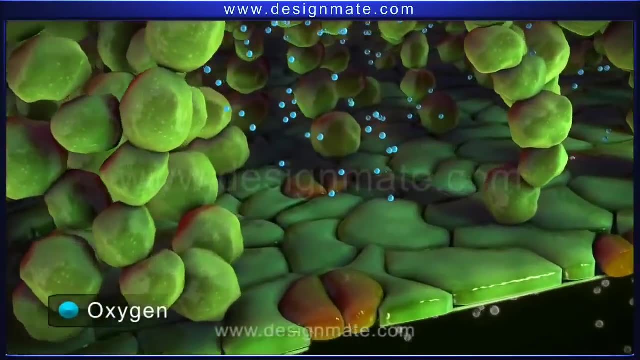 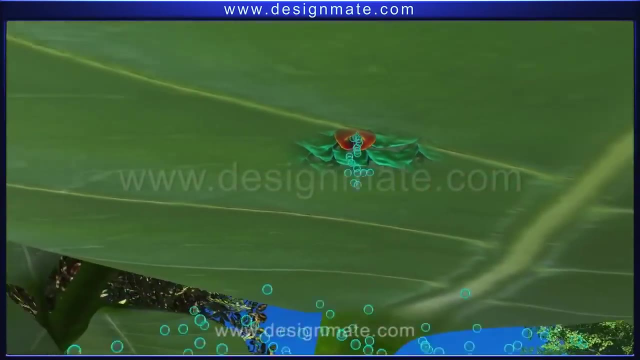 The glucose is transported through other specialized tubes to all parts of the plant, aiding in their growth. The oxygen present in these air spaces diffuses out through the stomata, So during photosynthesis, oxygen is given as the life-sustaining gaseous component of.